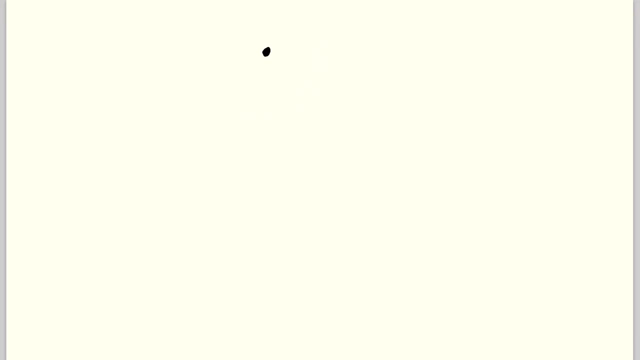 vertex and this is our graph. Then what is the degree of this vertex? The degree right now is zero and that's because there are no edges incident with this vertex. So the degree of a vertex is the number of edges incident with that vertex, which is the same as the number of. 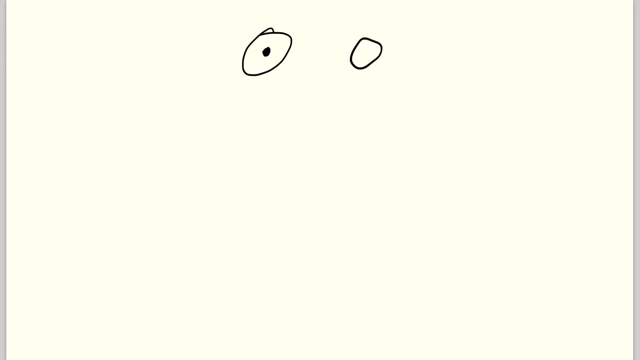 vertices this vertex is adjacent to, So in this case it's not adjacent to any vertices and thus it has degree zero. Then if we draw another vertex and we'll connect them with this blue edge, then the degree of both of these vertices is one, because this vertex is incident with one edge. 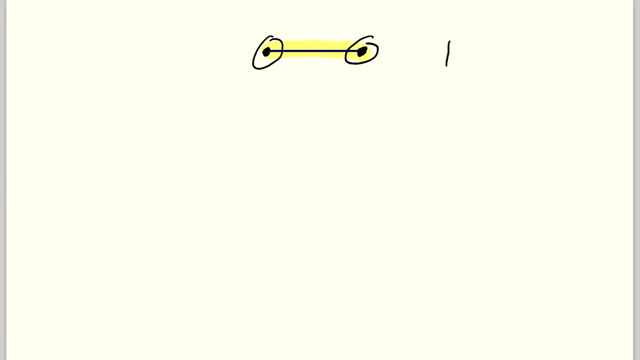 this blue edge here and this vertex is incident with one edge, of course the same edge as the other vertex, And equivalently they're both adjacent to one vertex, so they have degree one. And then, just for one more example, 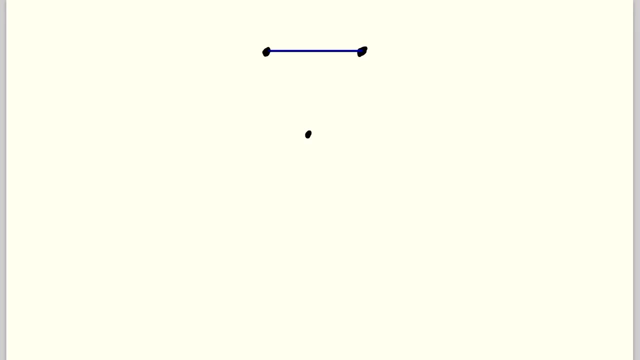 let's draw another vertex and we'll join this vertex to this vertex. then these two vertices here have degree one, because they're both adjacent to one vertex, this one here And again. equivalently, they're incident with one edge each. 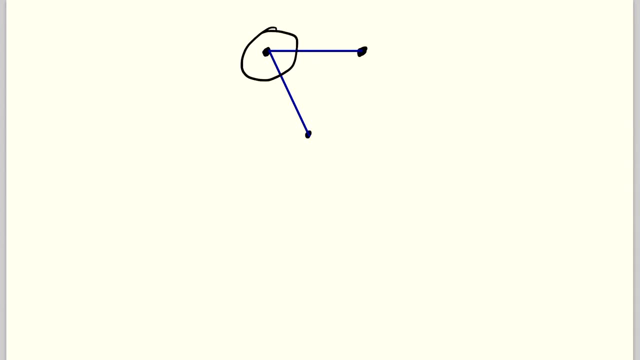 so they both have degree one. This vertex here, however, has degree two because it's incident with these two edges or, again equivalently, it's adjacent to these two vertices. The degree of a vertex is the number of edges incident with that vertex or, equivalently, the number of vertices adjacent to the vertex. 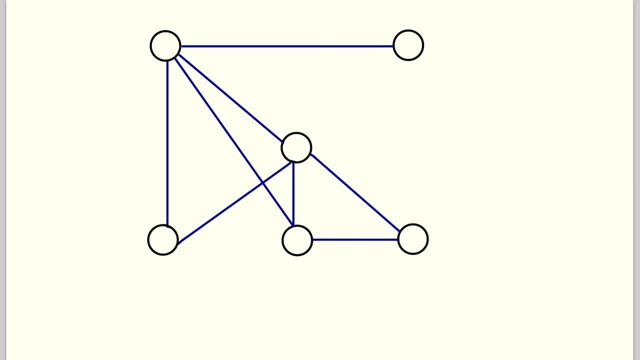 Now, here we've got a neat little graph, a fun exercise for us. We're going to look at each vertex, the empty circles, and inside the circles we'll put the degree of the vertex. So let's start with this one. here We see that has degree one, because it's only incident with this edge here. 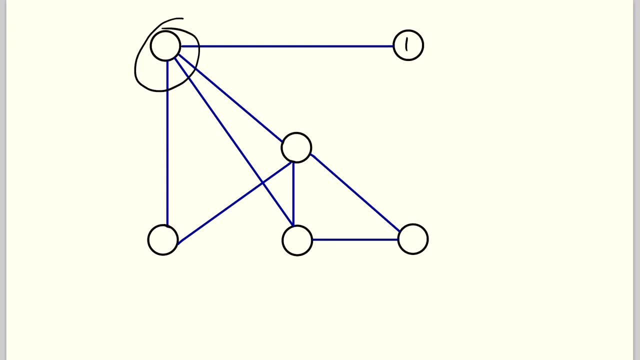 so we put that one in there. Then, moving on to this vertex, we see it's incident with one, two, three, four edges, so we'll plop a four in there. Moving around to this one down here, we see it is incident with these two edges here, so we'll put a two in there. This vertex here is incident with one. 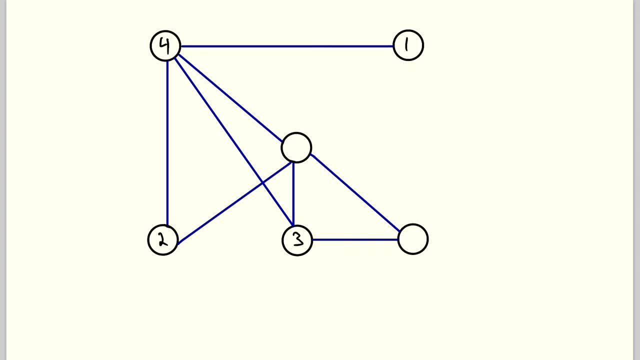 two, three edges, So we'll put a three in there. This vertex here is incident with these two edges, so we'll put a two in there. And then this vertex here we see is incident with one, two, three, four edges. 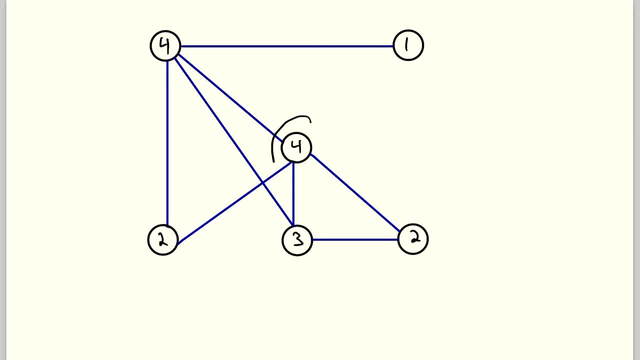 And so we put a four in there. And if we look at this vertex again, we counted up the edges. but of course you could also count up the adjacent vertices. It's adjacent to this vertex, this vertex, this vertex and this vertex. 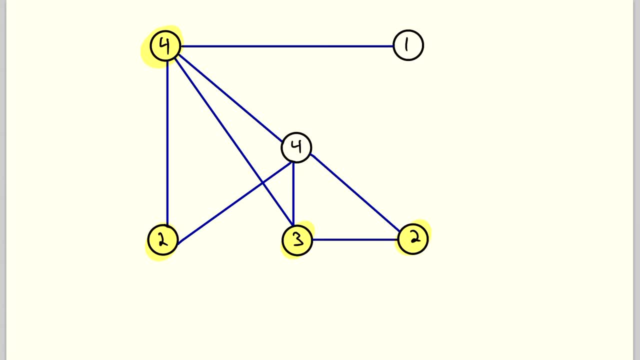 So it's adjacent to four vertices and of course that gives us a degree of four. So now that we've got the degrees of these vertices filled out, let's just talk about a little notation. Let's go through and label these vertices for starters. 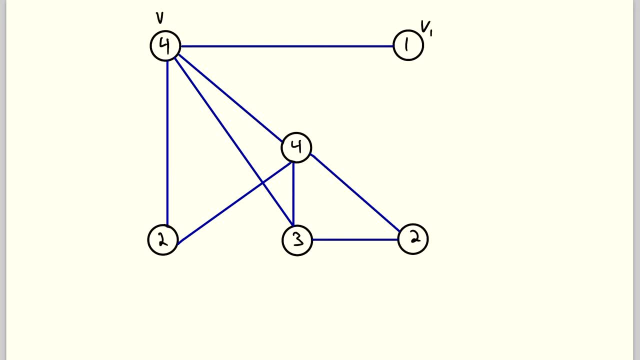 So I'm going to call this vertex v1,, this vertex v2, and so on. So I've labeled the vertices and let's call this graph g. Then we denote the degree of a vertex in this way: d, e, g of the vertex. 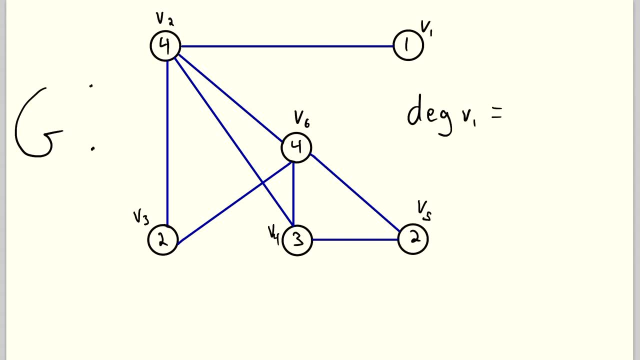 So here we've got the degree of v1.. We know that that is equal to one. We could also denote the degree of a vertex this way: d, e, g, and then, as a subscript, you put the name of the graph that the vertex is in. 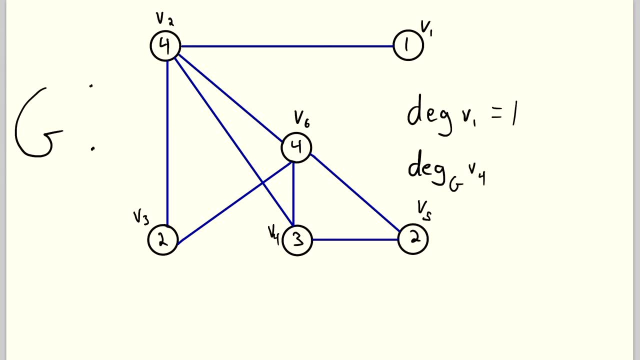 and then of course you put the name of the vertex. So let's look at v4, for example. So the degree of the vertex v4 in the graph g. we see that's right here and that has a degree of three. So you can write it this way: when the graph you're talking about 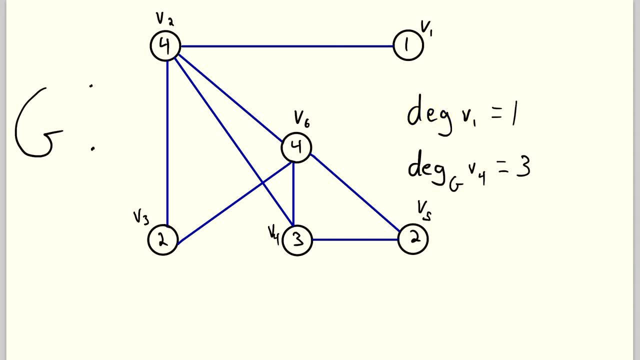 is clear, But if you're working with multiple graphs at once, it would be wise to use this notation with the name of the graph in the subscript, so it's clear what graph you're talking about. One other thing I'll mention is notation for maximum and minimum degrees. 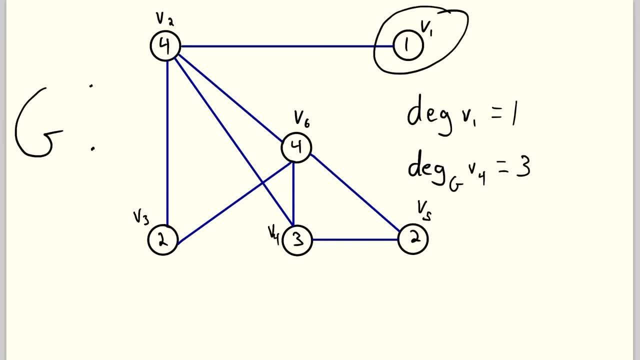 So the minimum degree of this graph is one, because that's the smallest degree that a vertex in the graph has, and we denote that like this: This is lower case delta of the graph g. So that's the minimum degree of G, which of course we see is 1, because this is the minimum degree of any vertex in. 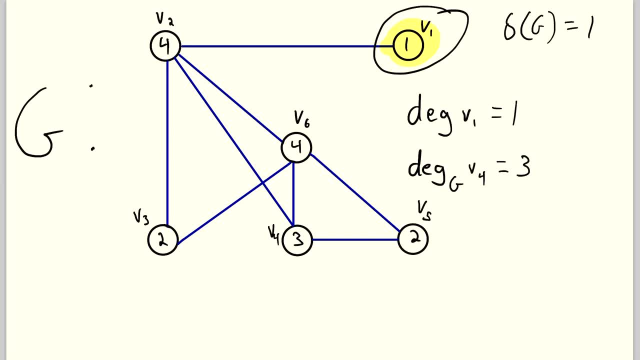 the graph G. And then, of course, we also have a notation for the maximum degree, and that is this: That's an uppercase delta of the graph G, and what is that equal to? We see that the maximum degree in this graph is 4, which appears twice, So we can say that the